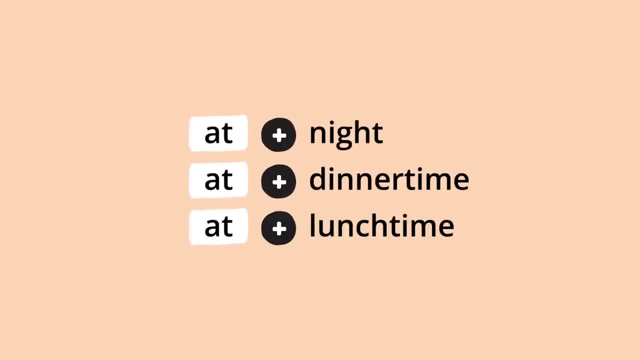 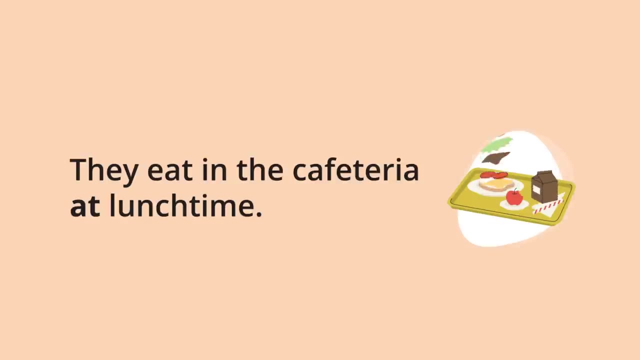 We also use at for other times. I watch TV at night. They eat in the cafeteria at lunchtime. We use the preposition on with days of the week. She has a job interview on Monday. We always play baseball on Fridays. We also use on for dates. 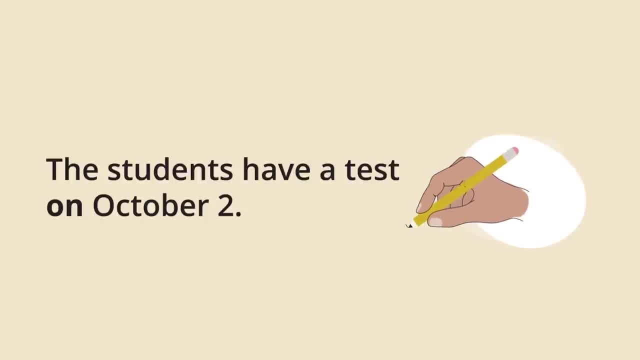 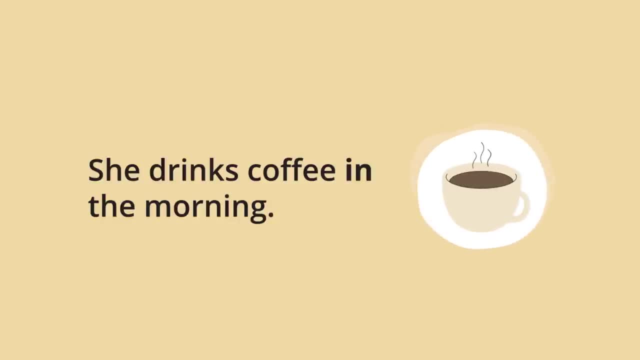 She drinks coffee in the morning. They go to the gym in the afternoon. We also use in for months and years. My mother plants vegetables in May. My mother plants vegetables in May. I graduated in 2019.. They go snowboarding in the winter. 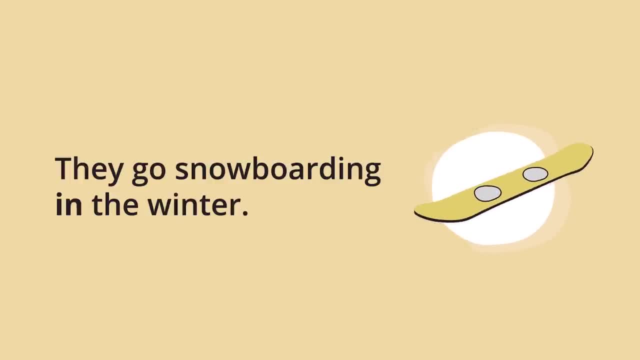 They go snowboarding in the winter. Look at the picture and say or write a sentence using a preposition of time. For example, We will take a trip in 2022.. Now you try. We will take a trip in 2022..